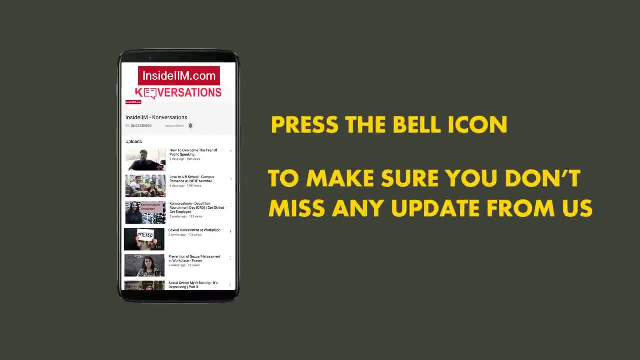 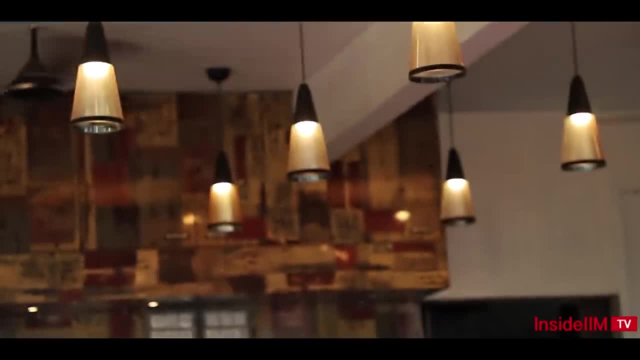 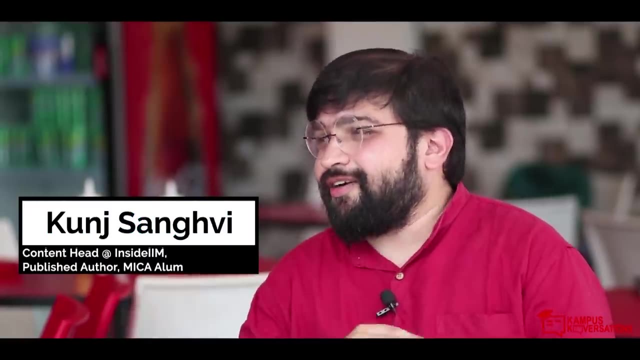 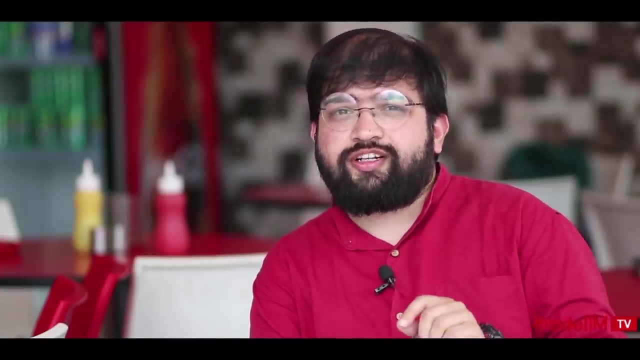 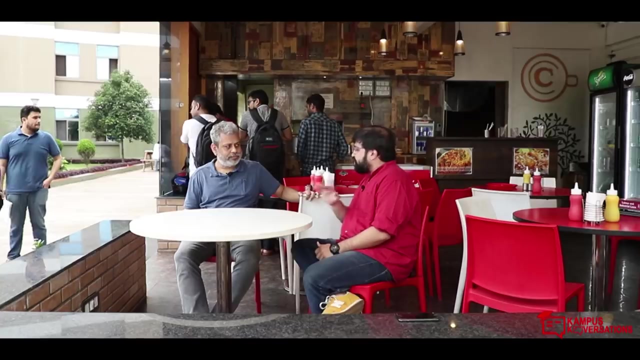 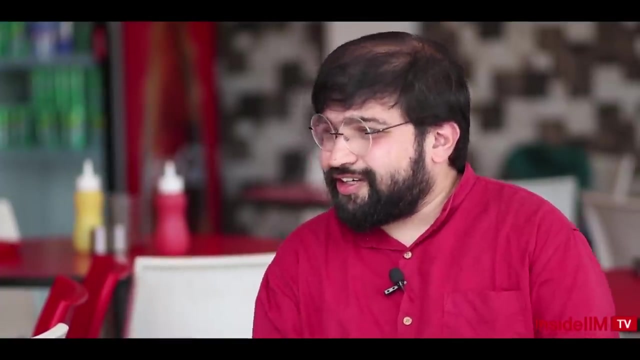 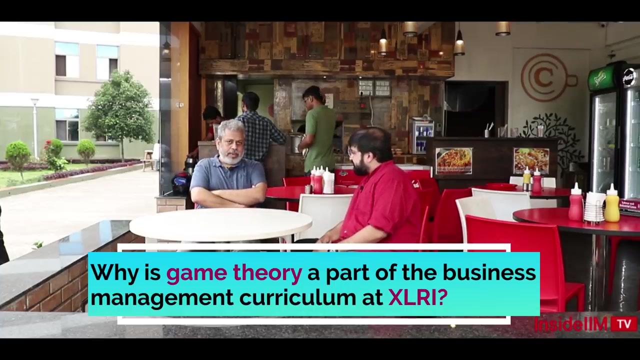 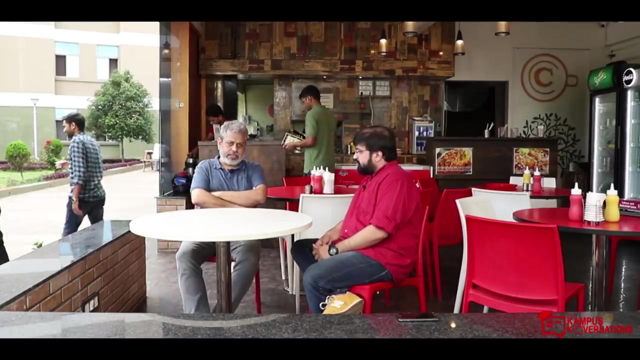 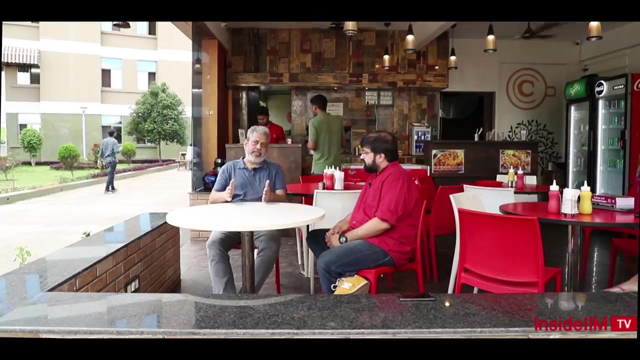 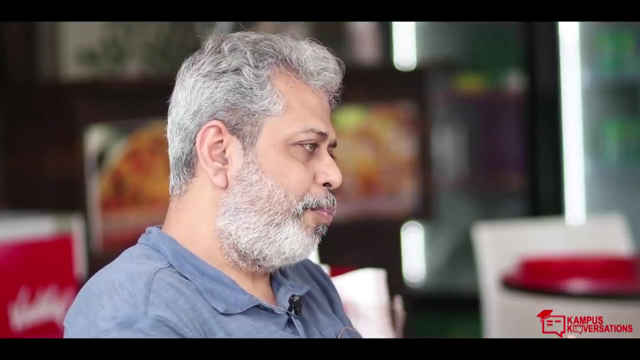 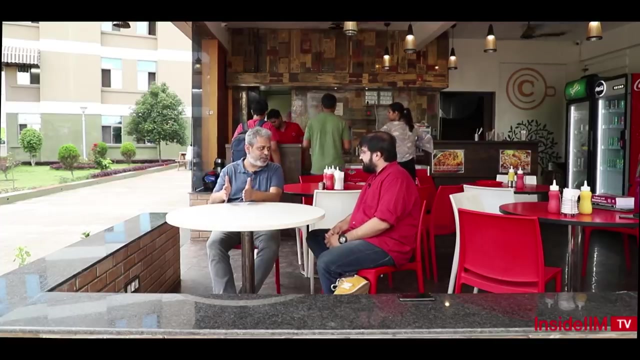 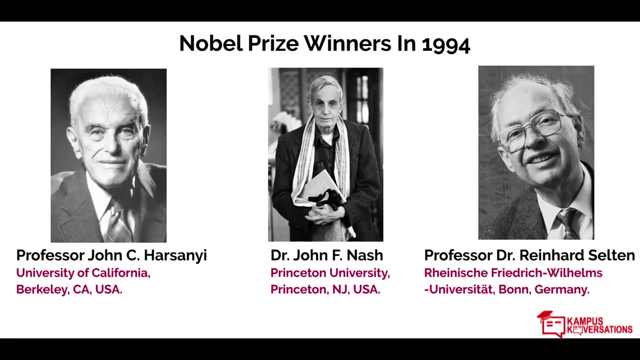 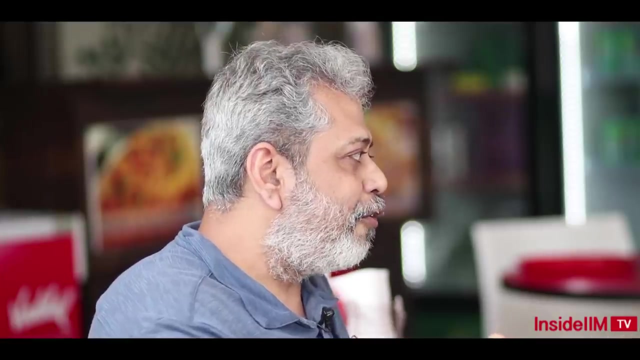 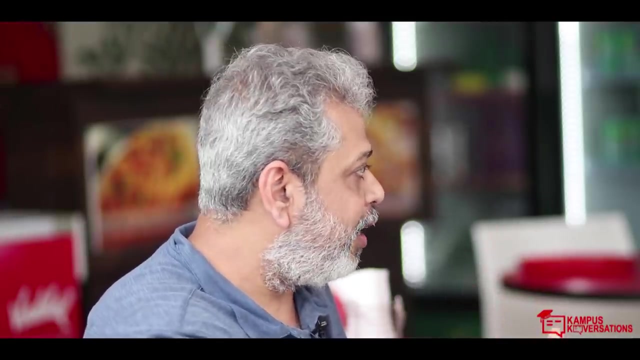 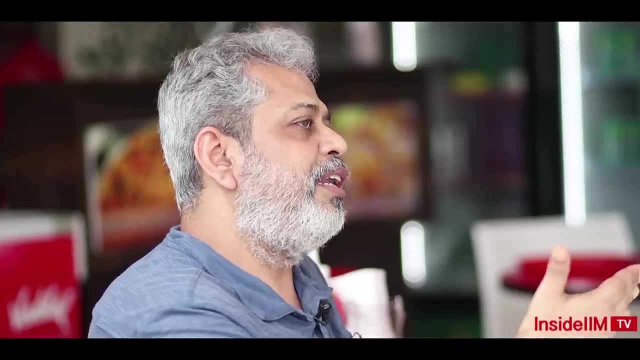 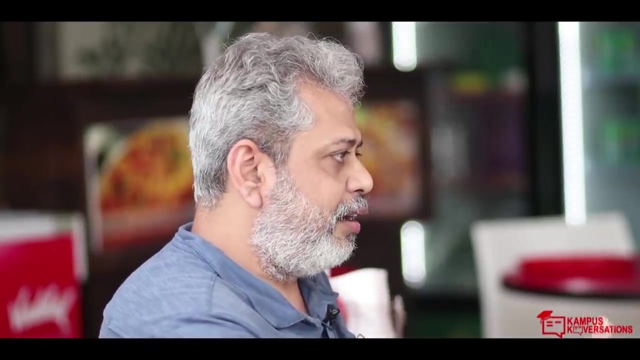 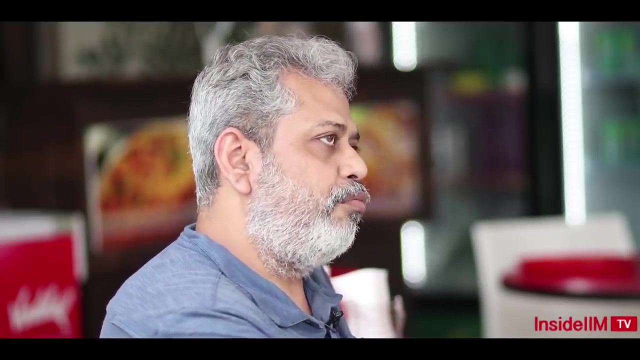 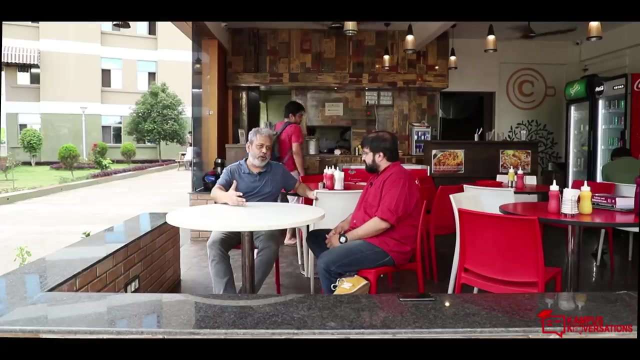 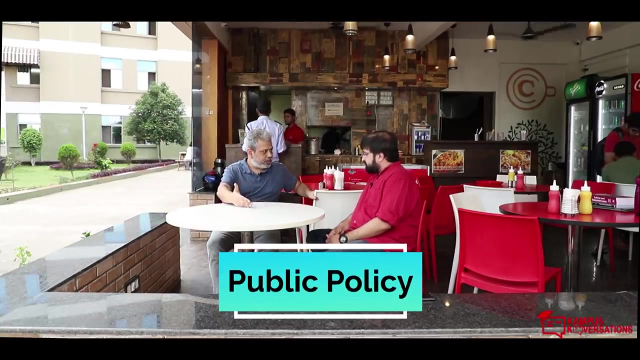 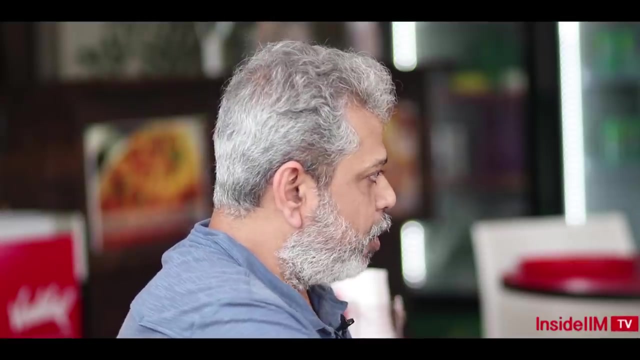 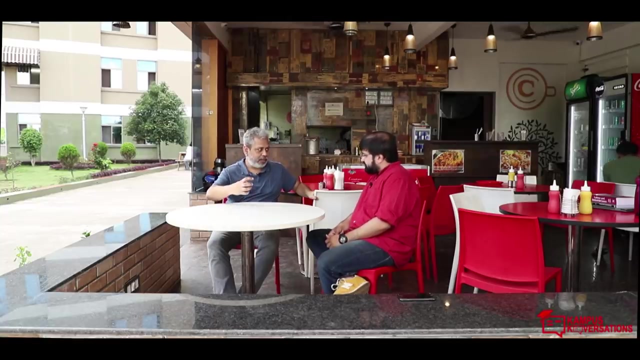 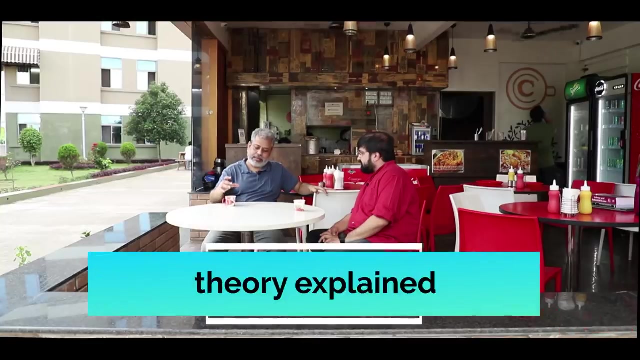 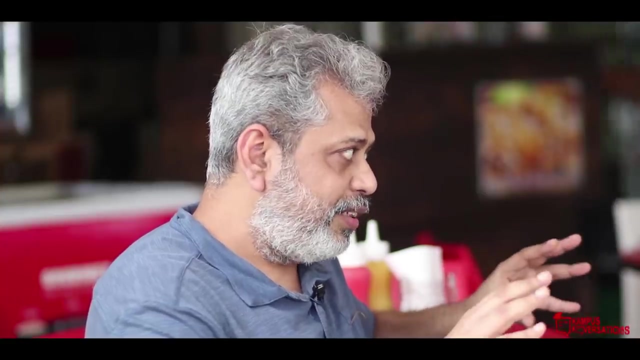 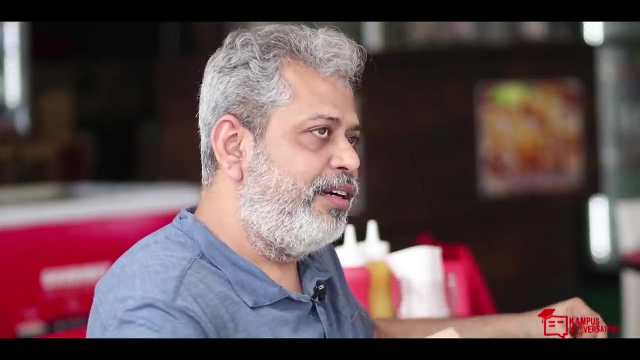 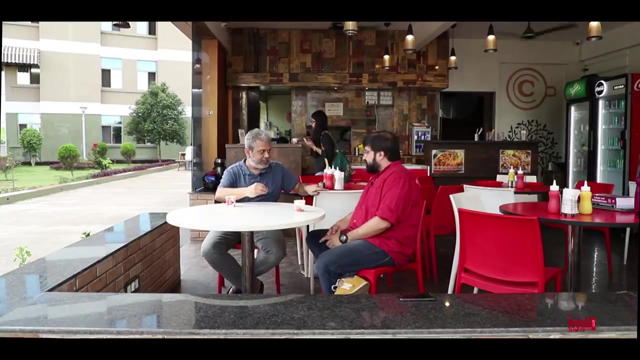 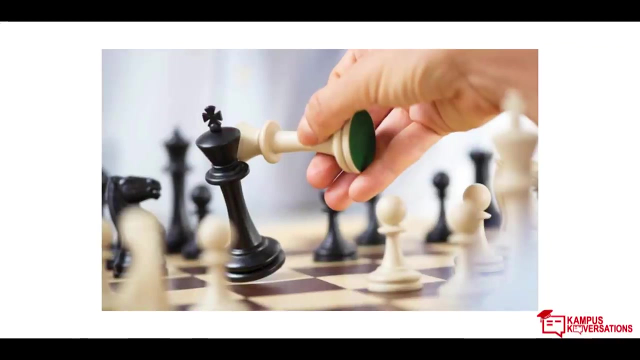 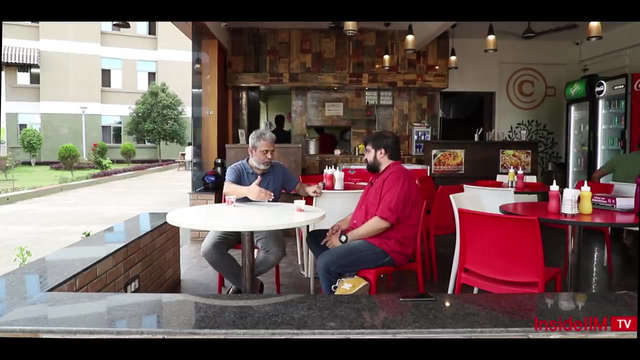 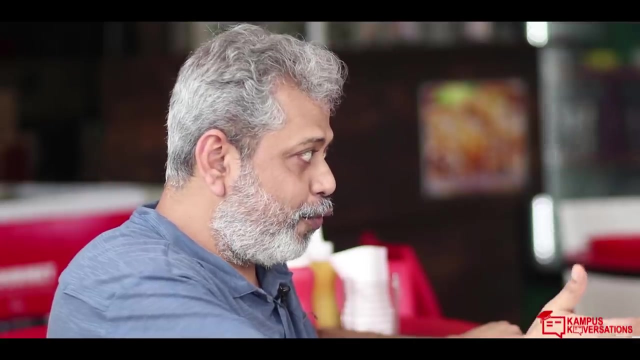 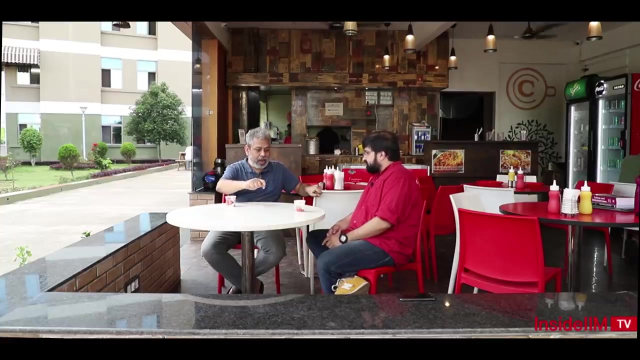 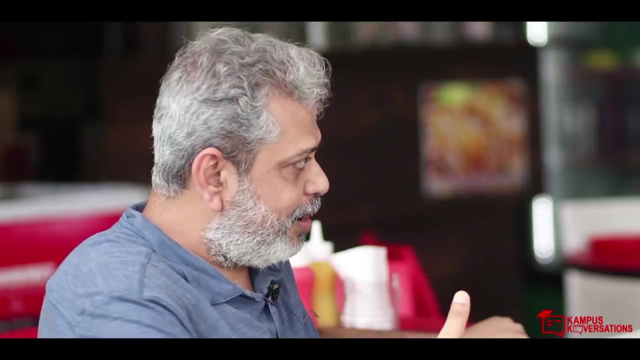 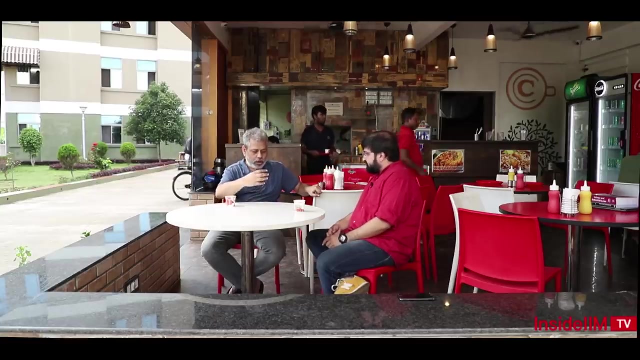 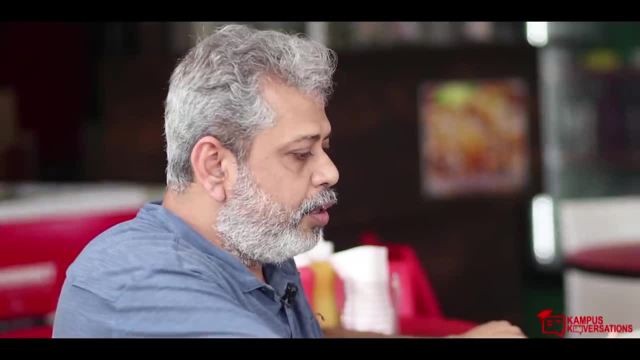 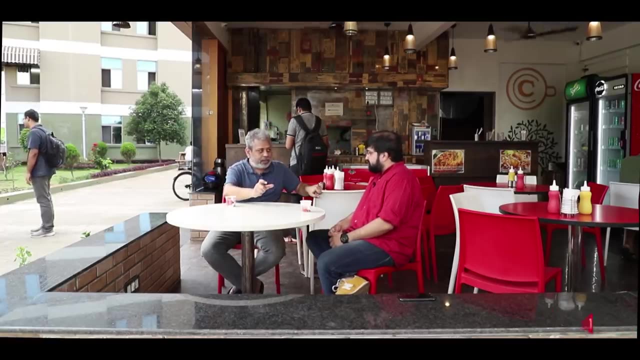 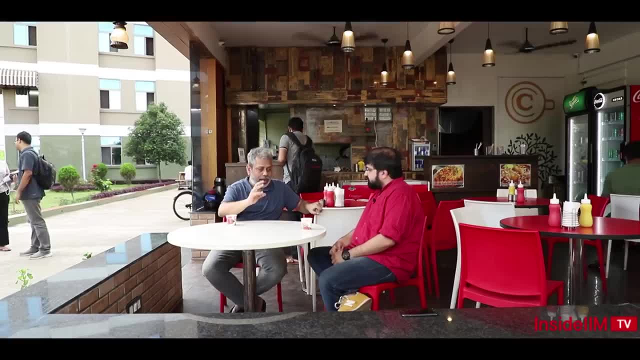 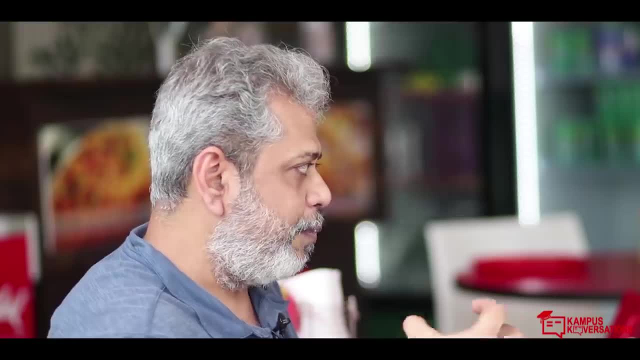 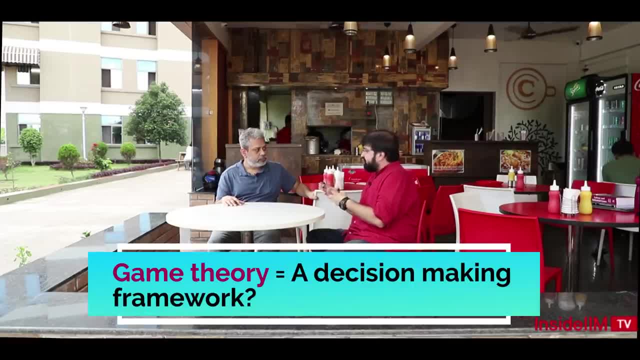 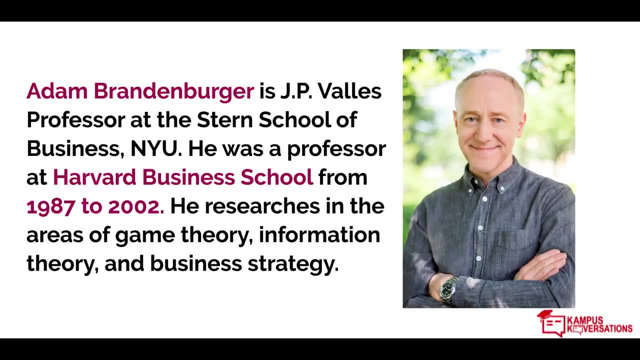 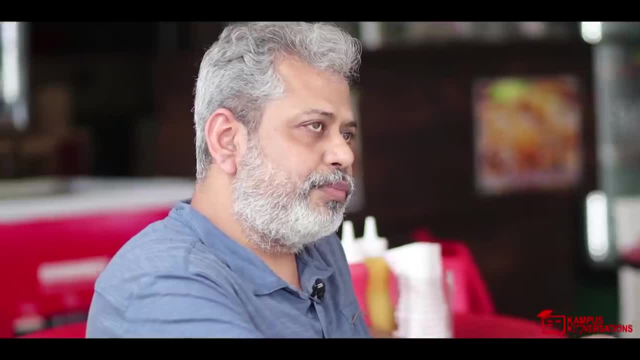 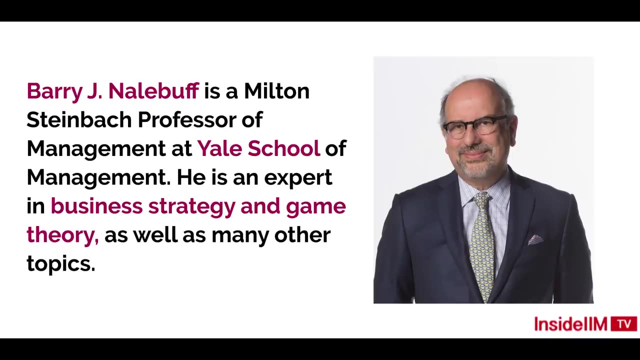 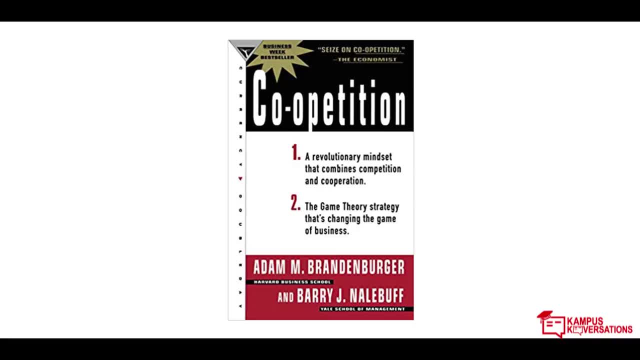 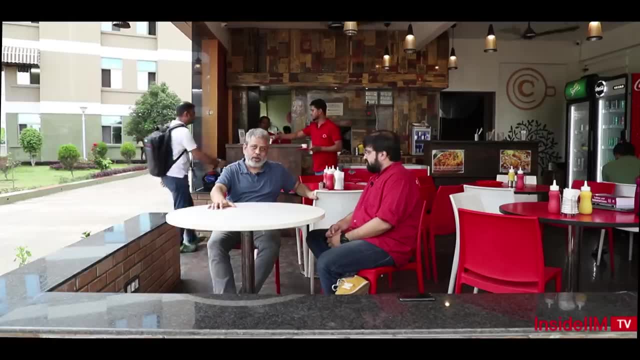 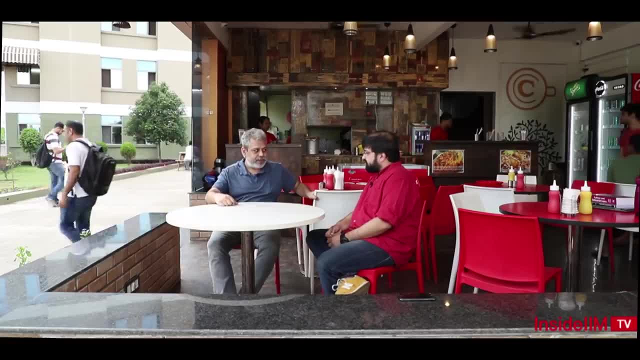 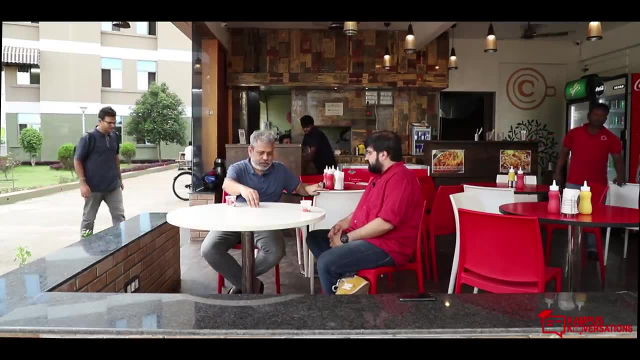 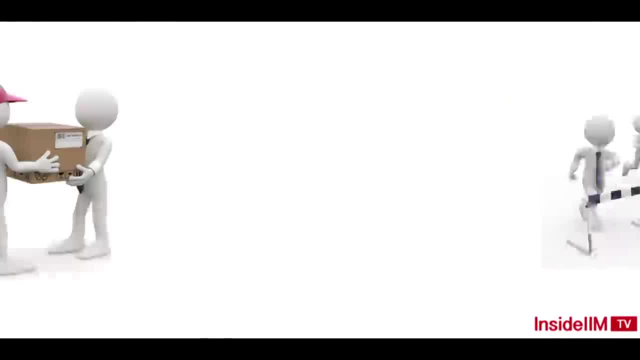 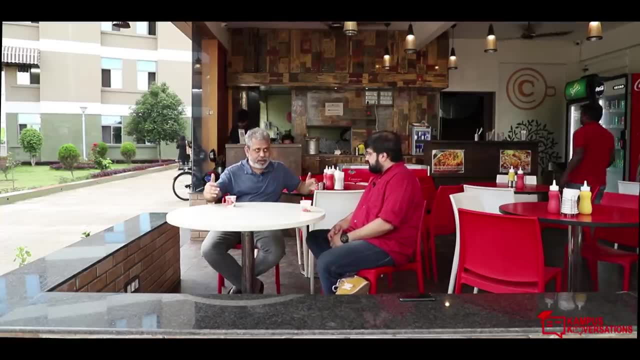 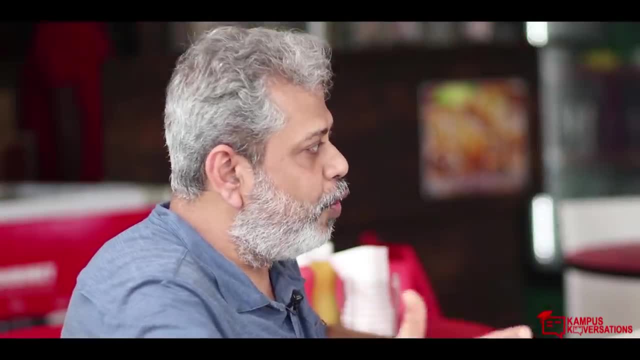 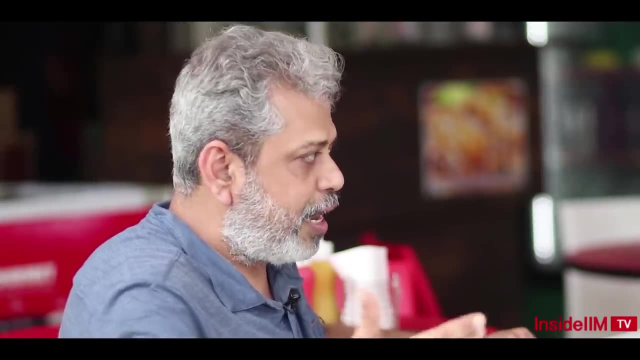 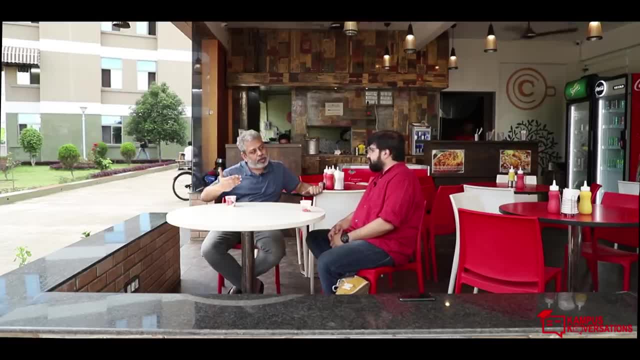 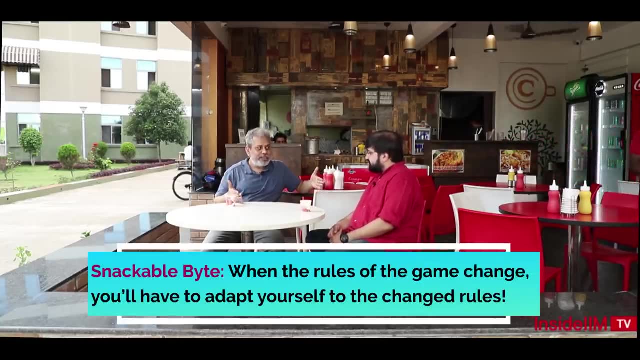 or something which is done by the government, and how do the farm respond to that? I mean okay. I mean you have to abide by the laws. you cannot. I mean so when the rule of the game changes. so then you will have to adapt yourself to the changed rule. right, and play the game, because the game cannot be played. 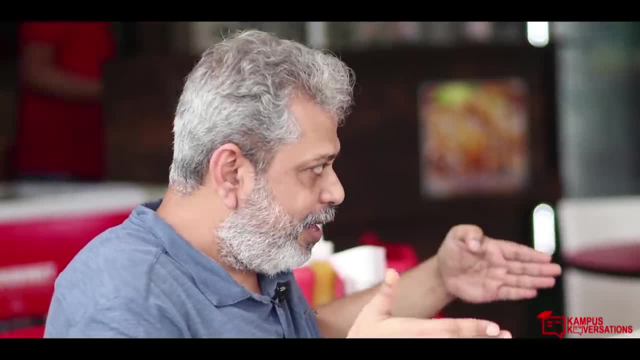 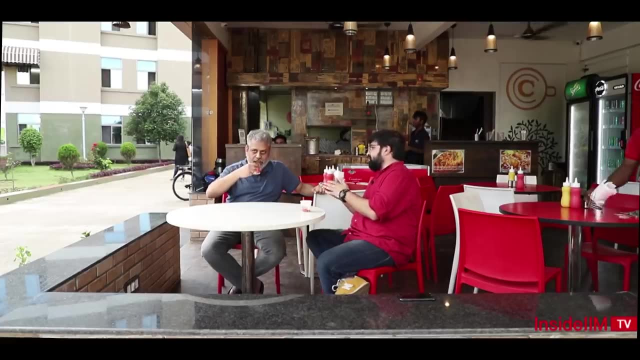 unfairly, illegally. you have to play it legal in the fair manner. let's take an example of uber. okay, okay, in the context of uber, can you explain this ecosystem where there are competitors and there are games being played with the competitor, there are suppliers, there is the government regulation and then there 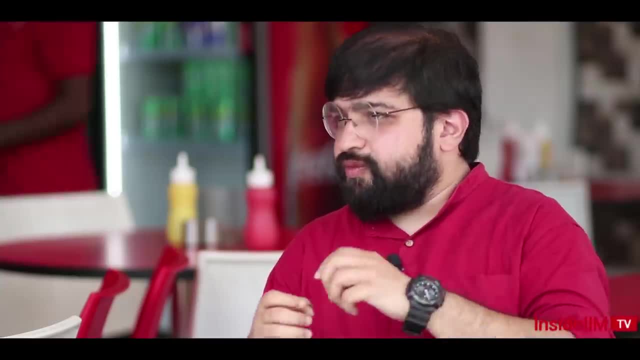 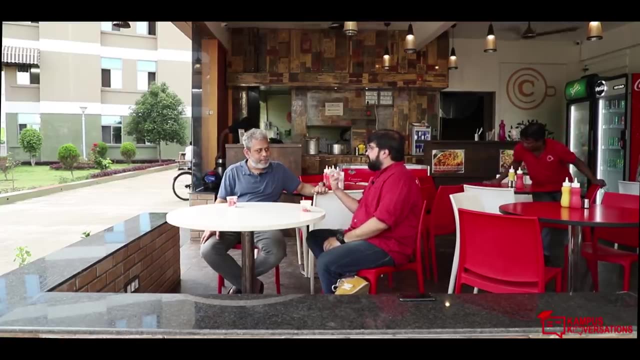 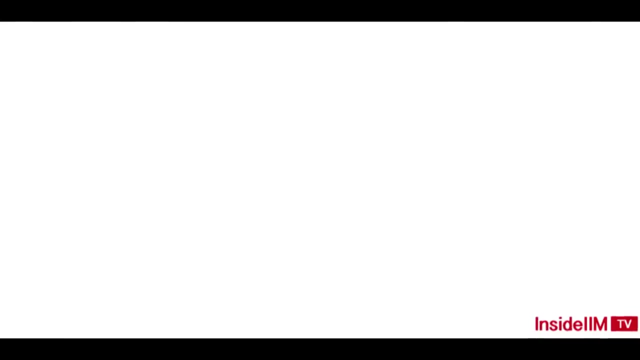 are, you know, vendors, like driver partners. with each of them, uber has a game equation going on, right, right. so how does that pan out? if you can explain with uber and as an example, maybe we'll better understand it exactly. I mean, uber fits very well in the framework of Brandon Berger, which is called a value. 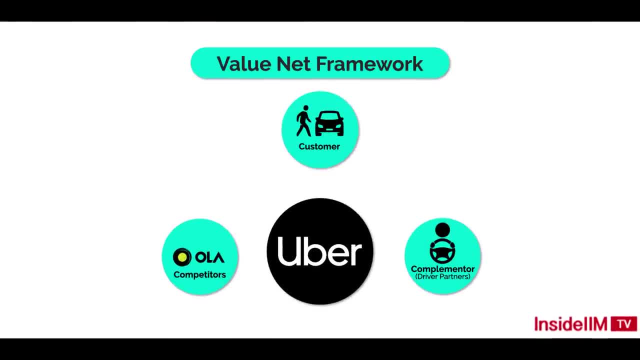 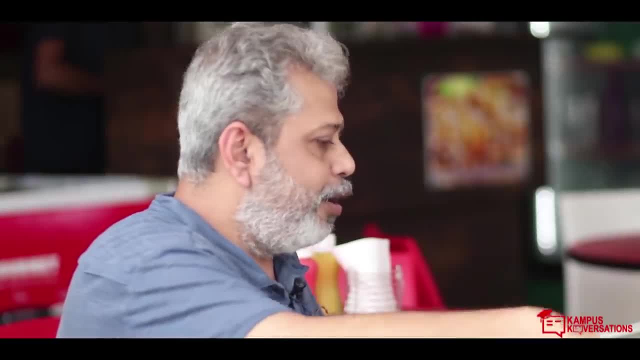 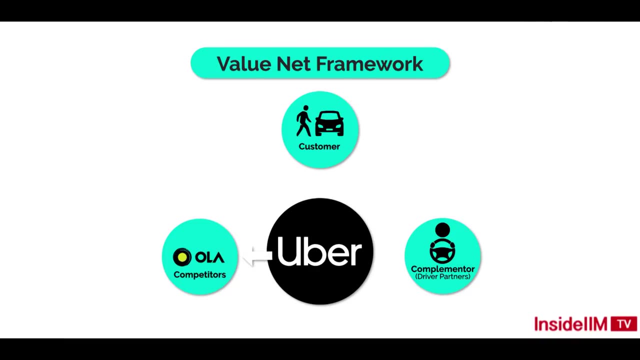 net framework. so, if you think of uber as the farm and if we are focusing with in the territory of India, right as the geographical region in which the decisions are being taken, their competitor of uber is essentially Ola. yeah, right, so Ola is the competition, their customers, who are the customers? 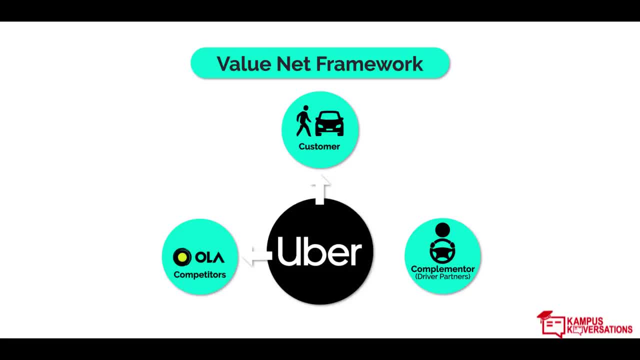 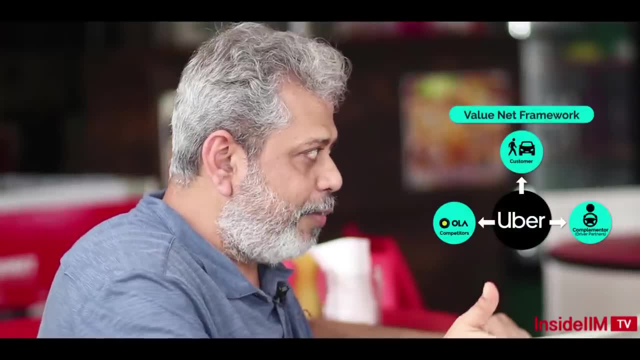 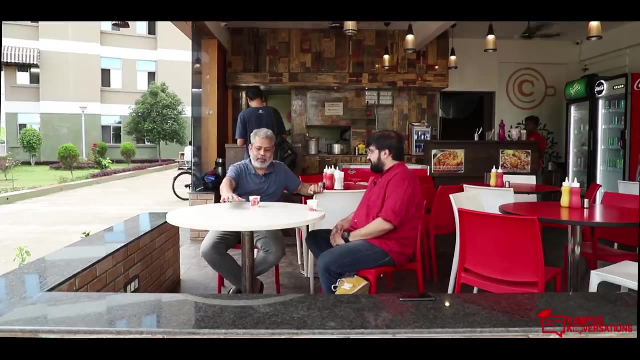 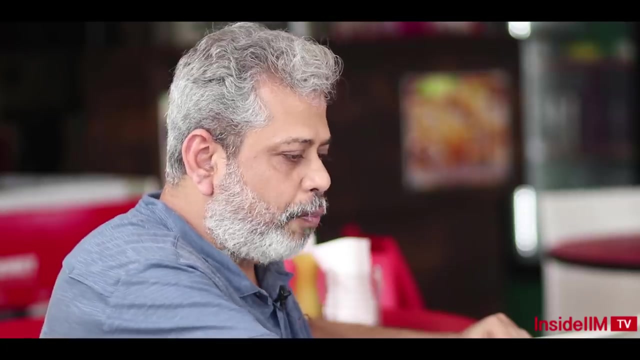 every commuter is basically a customer. okay, the cab owners or the drivers, who are? they are the suppliers or they are complimenters? I mean, this is a little tricky question, right, because uber is providing you the platform. right, it's a service providers of the cabs or the cab drivers. they are actually complementing this platform. 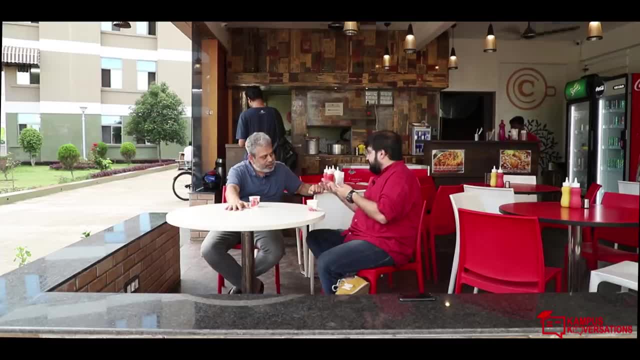 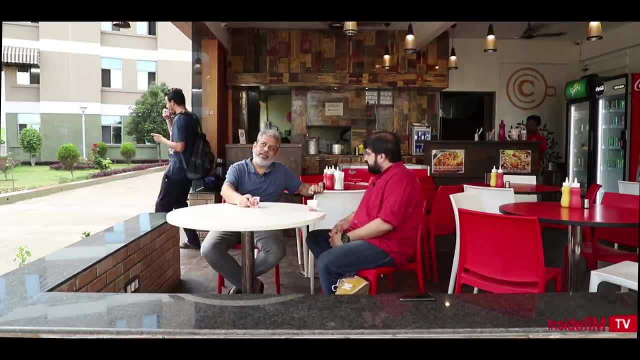 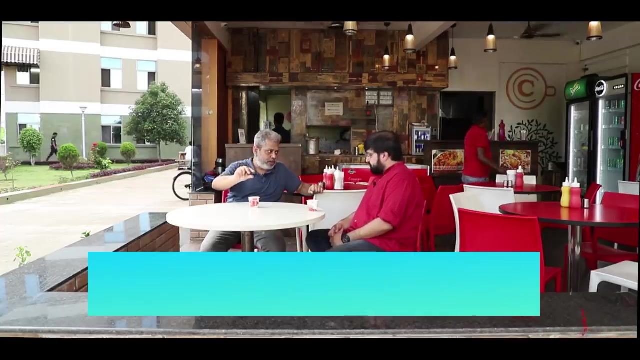 okay, right, but uber is so completely dependent on them. uber is completely dependent on them. maybe they are more of suppliers than complementary product providers. see, I mean supplier. it's not exactly the way we visualize a supply chain. okay, in a supply chain, what happens? farm one pumps, product those as input to another farm. 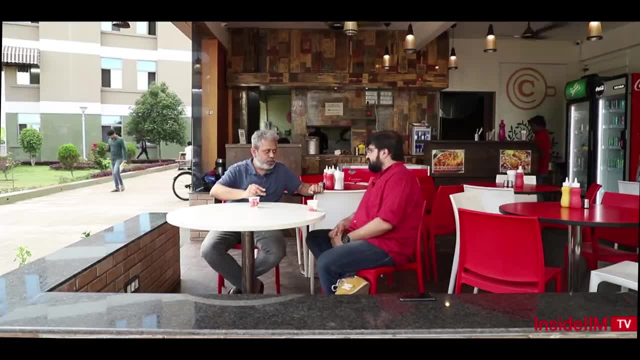 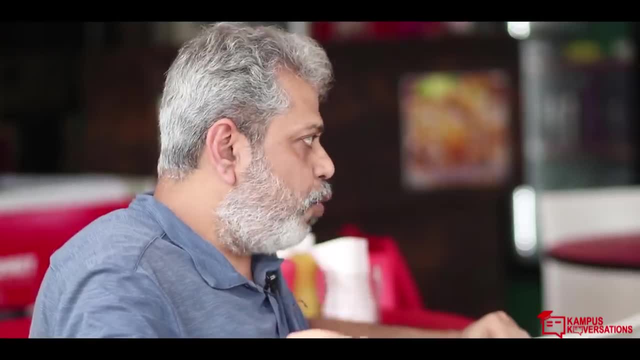 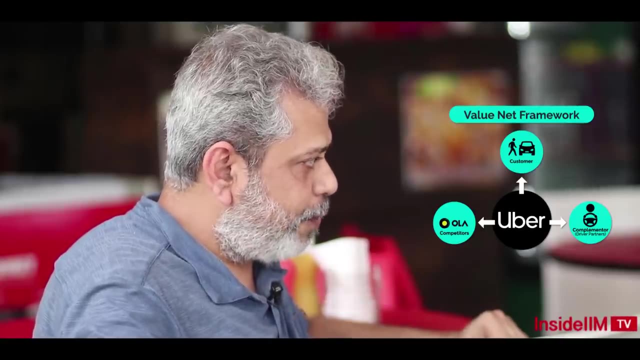 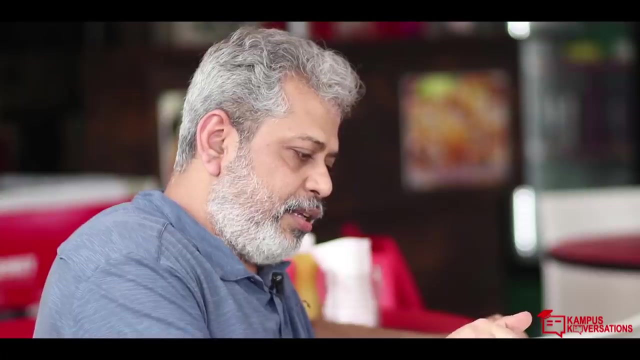 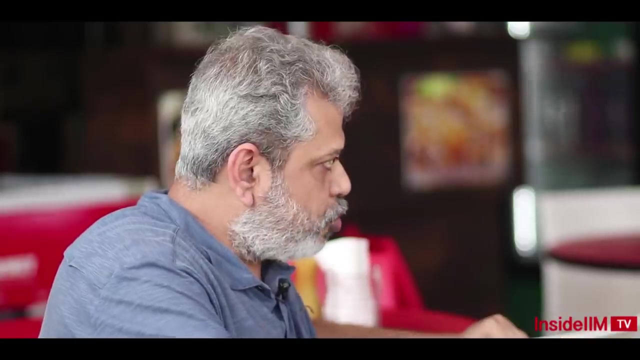 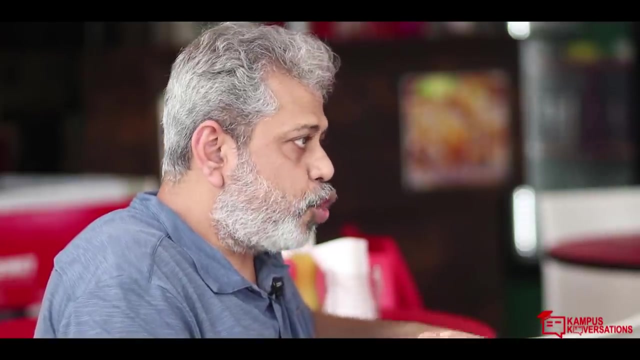 right, and then they make another product which goes to another form or to the retell outlet. okay, now, in that sense, this cab owners or the drivers are not really suppliers to uber, they are actually complementers. now, here the game is. I mean, two games are there One? is that the pricing game? Okay, So Ola is following a particular pricing strategy. Uber has to follow a device, a pricing strategy, in order to counter Ola, to increase their market share. So how do they do that? 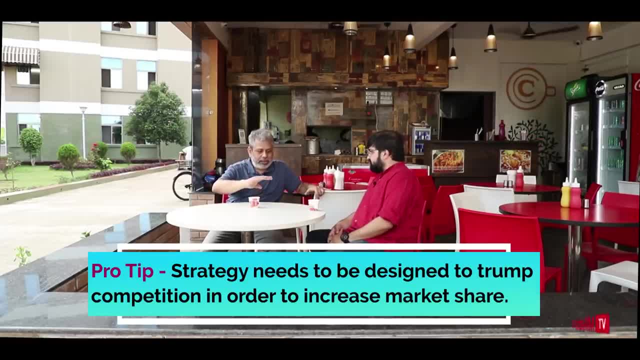 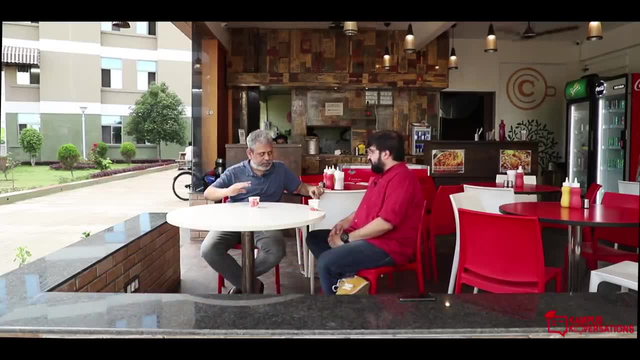 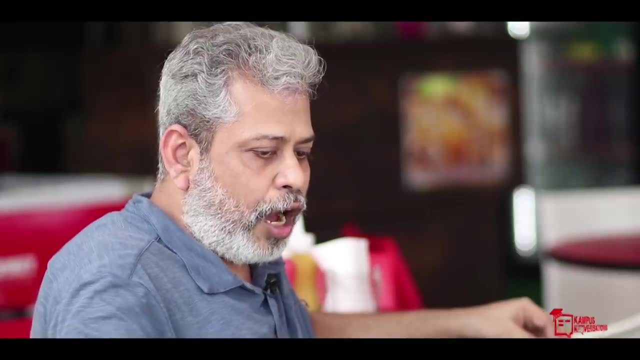 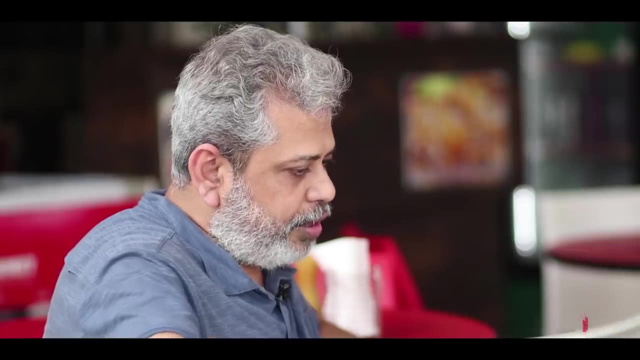 Okay, This pricing strategy is a little complex because this price varies with time, depending on the demand. When the demand is high, they increase the price. When the demand is low, they reduce the price. So that is one aspect. But then again, the competition aspect is there, Yes. On the other hand, how much do we pay to the cab owners? How much do you pay to the driver? So, the complimenters: There is a game between the complimenters and Uber, Because these complimenters can also shift to Ola. Let's not forget that. 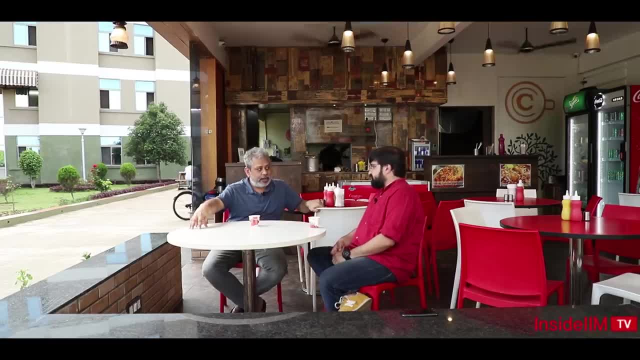 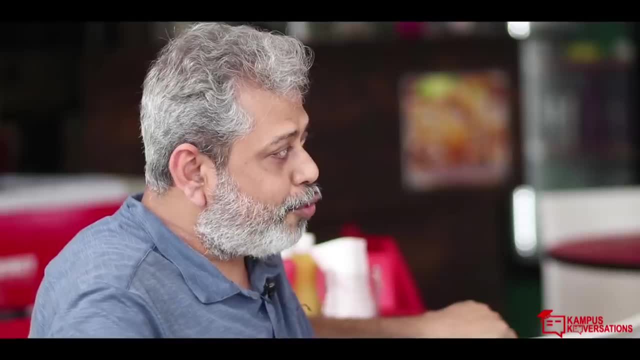 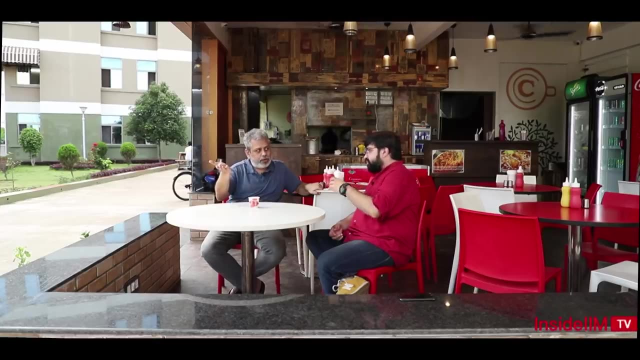 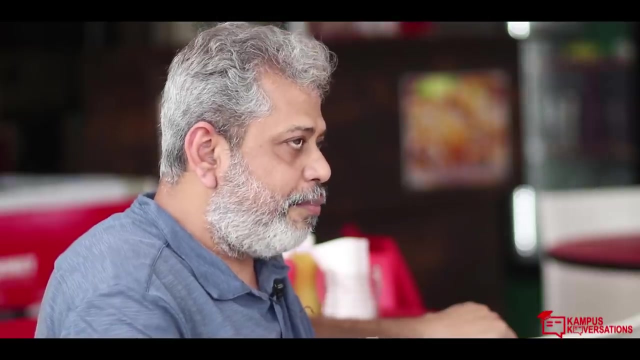 I mean, suppose I own a car, Now I can run that car as an Uber cab as well as I can run it as an Ola cab. I mean that is highly possible. I mean you will have to also incentivize them to stay with you, because otherwise what will happen is that peak hour. I mean you see that the competitors cabs are all around but your cabs are not there because you don't have enough cabs, I mean in the metro cities. I see these days Ola cabs are difficult to get. I mean, say, when 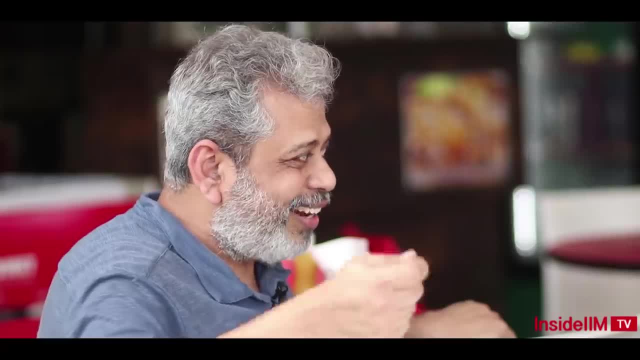 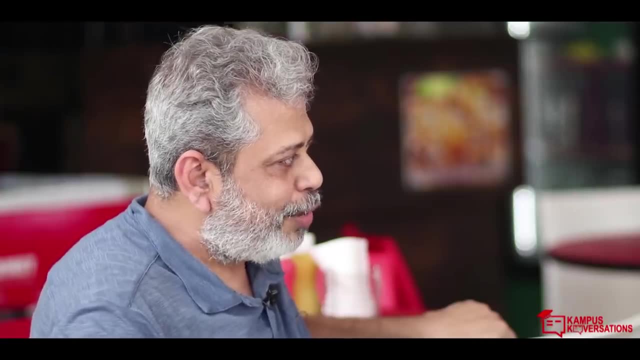 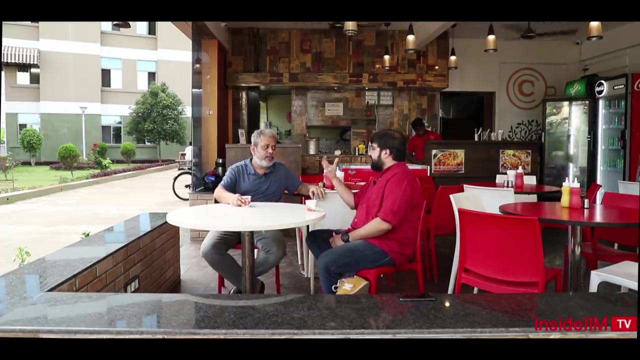 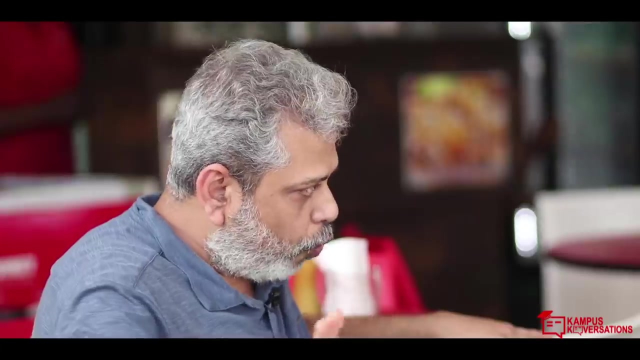 there is a high demand, I mean Uber cabs are more easily available. That essentially means Uber have actually captured more of those complimenters, that is, the cab owners. So that is why there are lesser number of Ola cabs. So Uber has got the incentive structure right. Possibly- I did not study it in depth- Yeah, but in that short term situation that's what it means. It looks like that they have incentivized the cab owners to stay with Uber rather than to move to Ola. Right, Sir? how does the government 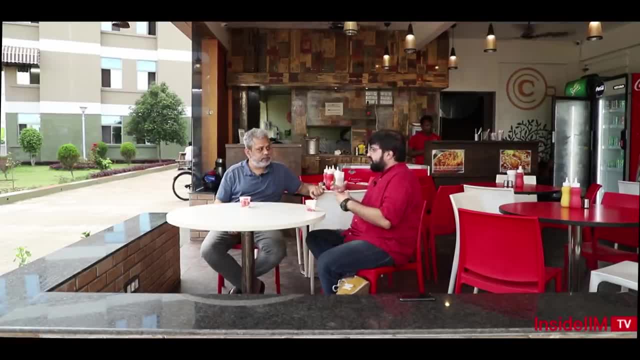 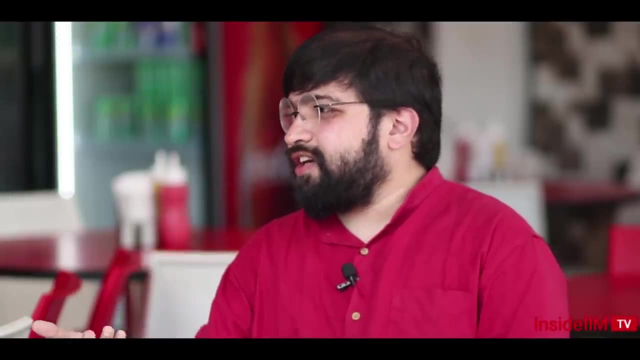 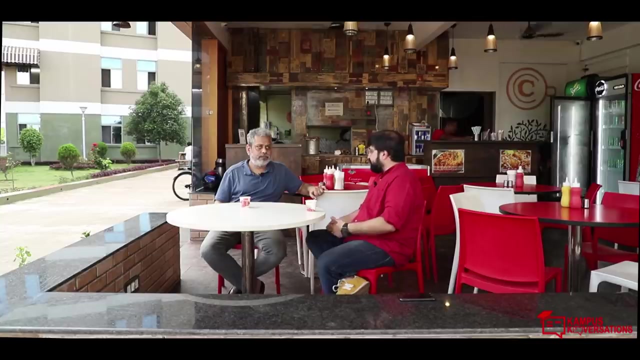 regulations play out for someone like Uber. Like, what game does Uber play with, say, the government? We see often that you know there is a push from the taxi unions and the auto unions to put a cap on where Ubers can be parked or what can be done, and there are strikes in big cities because they want to push government regulation to ensure that Uber, you know, does not take over the market. So is there a game again there, also with government regulation plays with Uber? Essentially, this is an economic problem. Right That? because 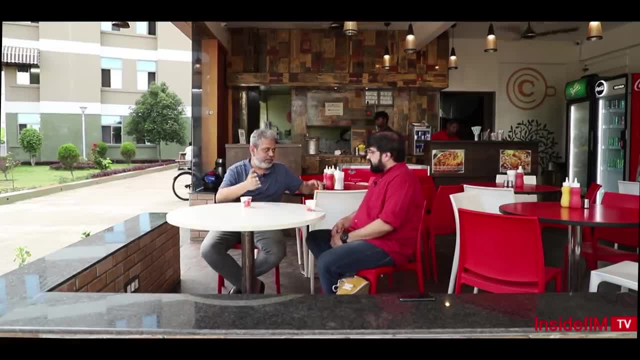 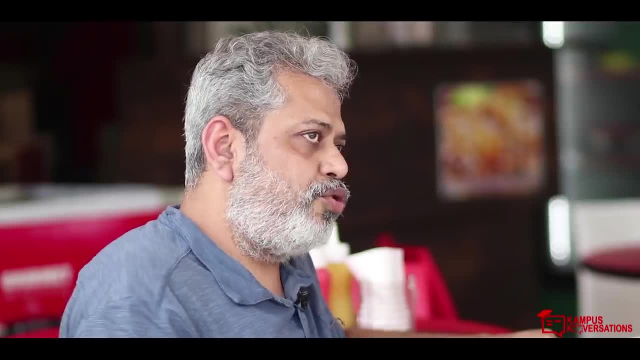 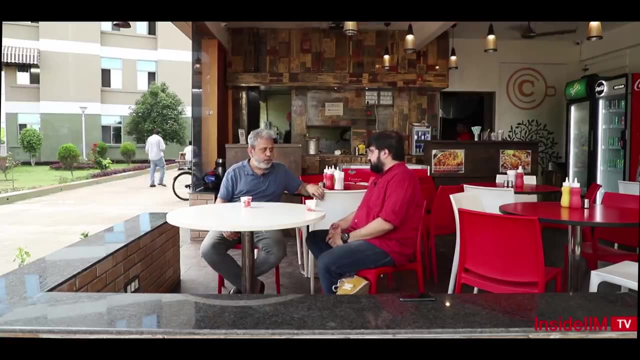 of Uber or even Ola, I mean any of these taxi companies they have done, I mean through their pricing and through their expansion, I mean they have actually created a scenario which results in loss of livelihood for, say, auto drivers, Big cities, I mean: you have these yellow black cabs. I mean now actually many of them are also running as an Uber cab or an Ola cab. 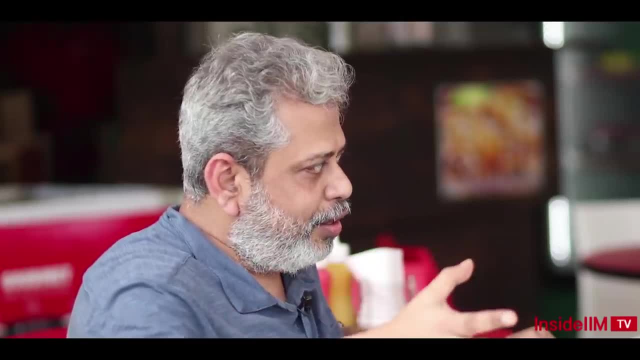 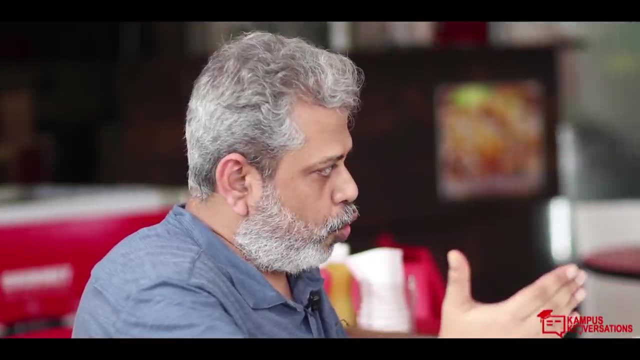 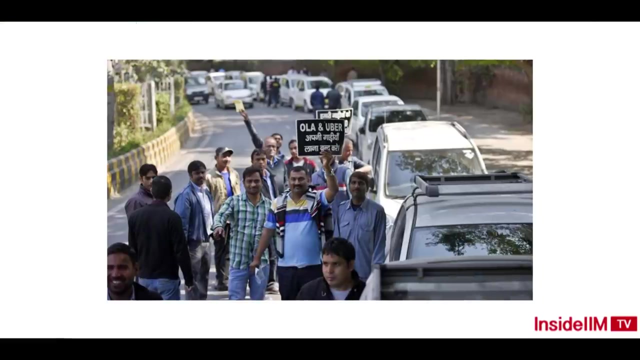 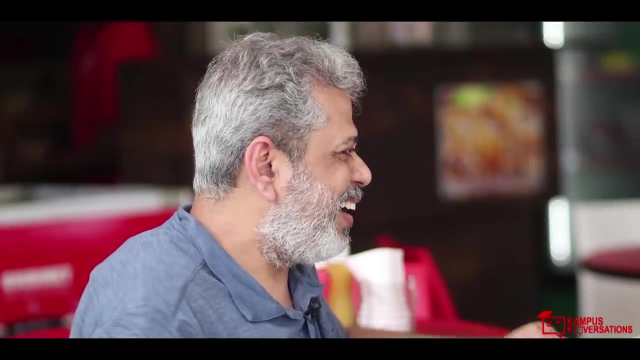 I mean so the so initially, when this app based taxi companies came, of course there was a backlash. Right Say, for example, auto. I mean, I know that in Lucknow auto rickshaw drivers actually went and growled Ola office. they did not want Ola to run. I mean, of course, I mean technological innovation, the progress cannot be stopped. But yes, I mean, in the transition period a lot of people lose their livelihood, Right, 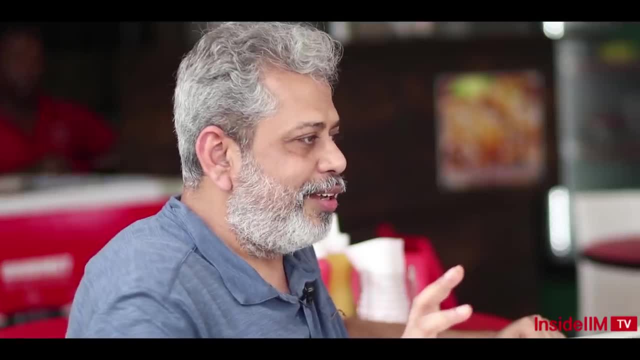 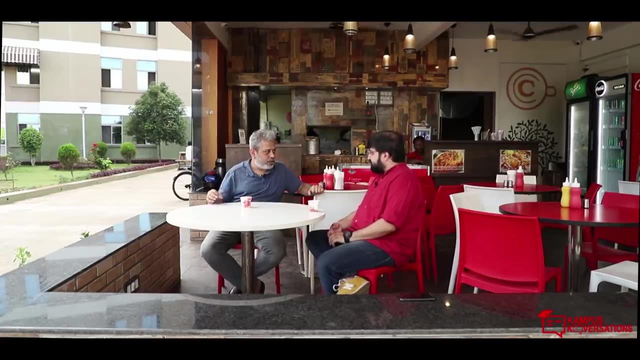 But government regulation, if you come to, it's a another story, because I mean, if you think of voting as a game, I mean how common people will vote Right. So I mean, on one hand, if you do not appease the auto rickshaw drivers, I mean, then you are creating a livelihood problem to a section of the society. and who might turn against you? 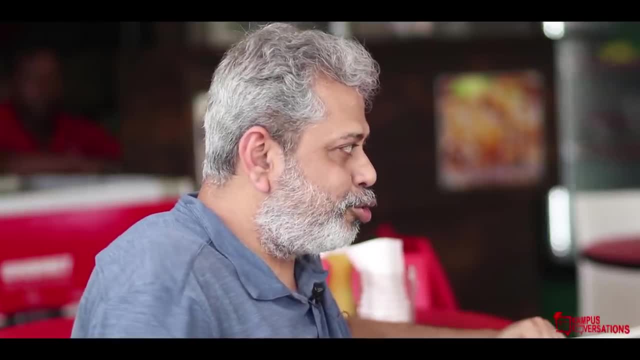 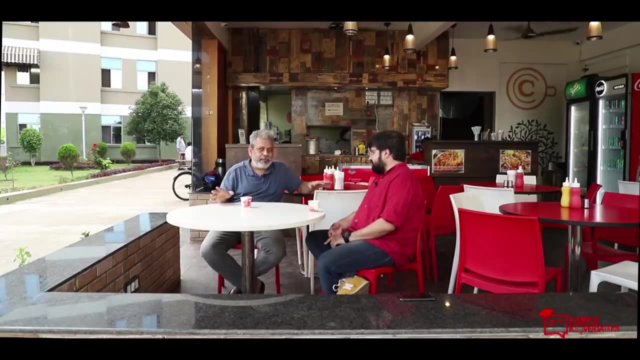 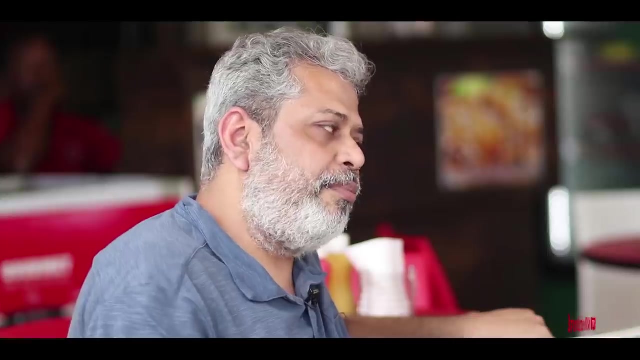 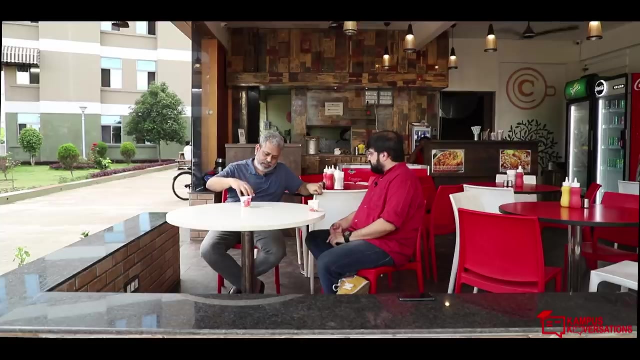 And might not vote Yeah. But on the other, it's a double edged sword, because customers might be unhappy if you are restricting Ola and Uber. So I mean, I mean, government did not really intervene in this domain as yet, Right. But yes, public policy, when you say designing a mechanism, has a lot, of, a lot of things going to it. One is that whether the mechanism that I'm designing will work or not, That is one thing, Right. So for that we use game theory, Right. 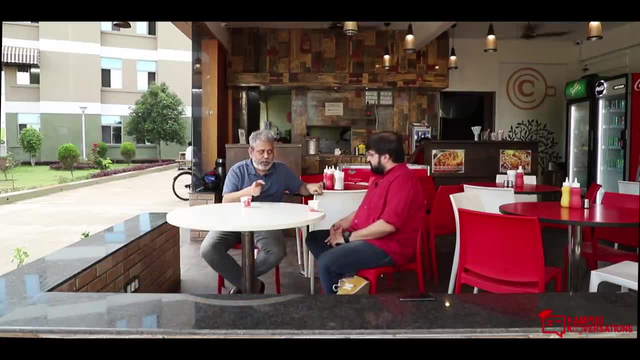 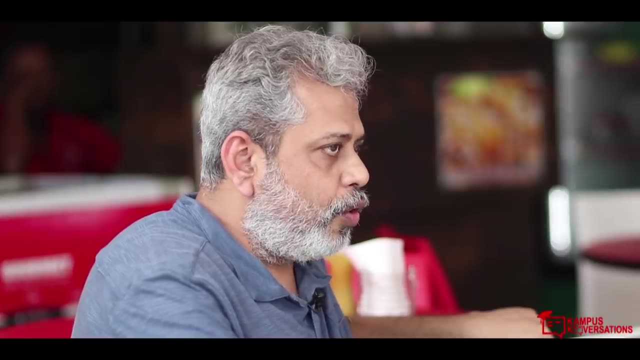 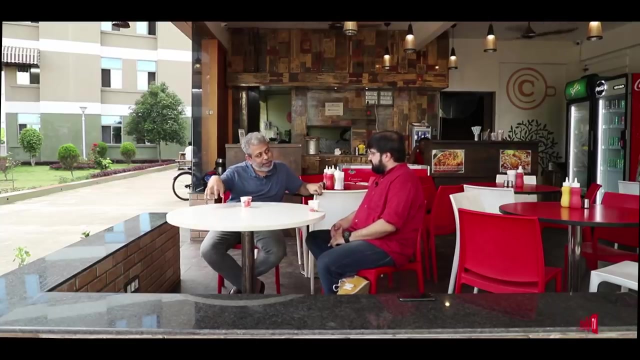 So because when I design a rule, whether people will find a way to game the system Right And and and bypass the rule, That is one thing, Right. Secondly, even if I can implement it, then what would be the ramification of this policy on my vote bank? because I want to come back in power as a political party, Right? So, so, so that also, that equation also needs to be taken into account. So you're saying that, say very big decision like 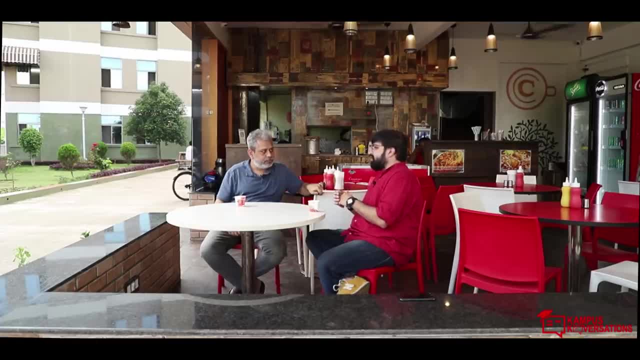 monetization is taken, or the GST is implemented, or even the odd, even policy that is laid as in that is rolled out, in Delhi, for example. Each of these situations would have been, you know, looked at through the game theory prism before deciding how you want to structure that policy. Not all of these say, for example, GST. OK, I mean, there is no game here. It's basically a mechanism of tax collection. So which process is more? 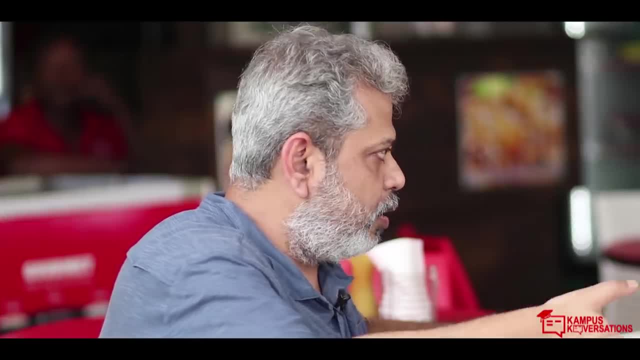 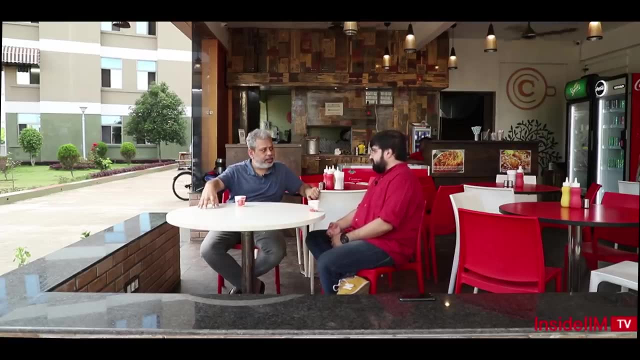 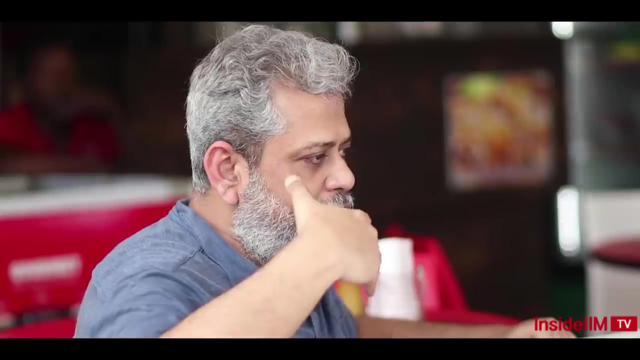 efficient, which reduces the different bottlenecks that exist in the system. It's a different decision. It's an economic decision, Right, But does not strictly rely on game theory. But there is a backlash of the public that is also there in that situation, Right? So again, the vote bank and all that. So voting game is another game, Yeah, But then again, the government interaction with the public, Right. I mean through those interactions when they campaign, they try to 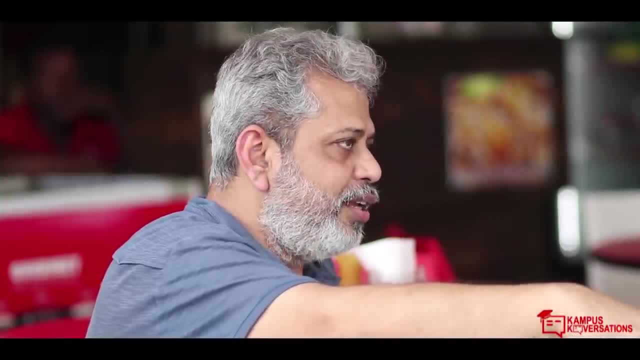 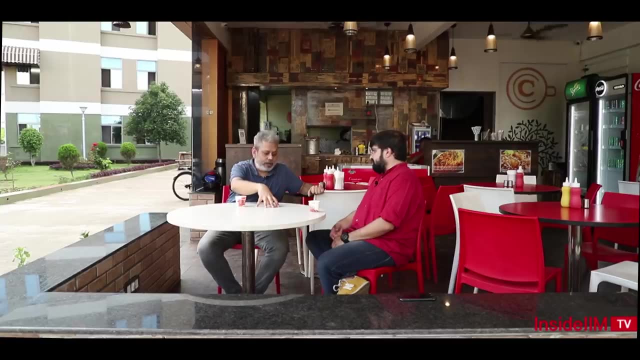 convince the public in the way they want to do Right Right. So, for example, if you are talking about demonetization, it has nothing to do as such with game theory. It's macroeconomics. When you are removing a certain amount of currency note from the system, there are economic ramifications of that. That is one thing. But then again you are telling people that we are doing this to reduce black money. A lot of people have gotten too rich. Yes, They have black money, which is basically untaxed income, So we are trying to remove that.